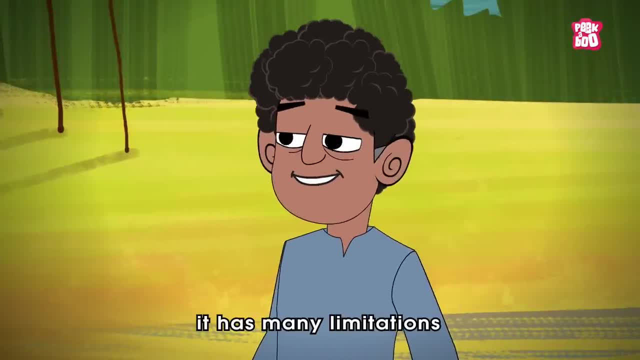 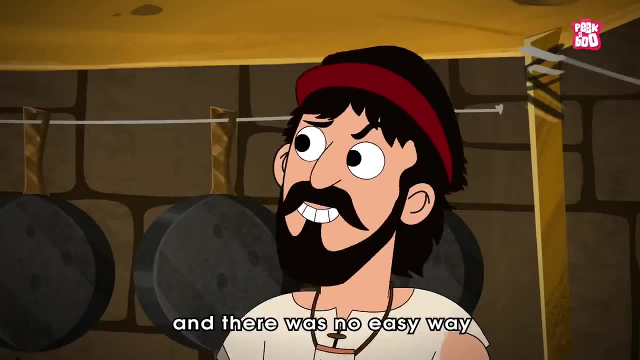 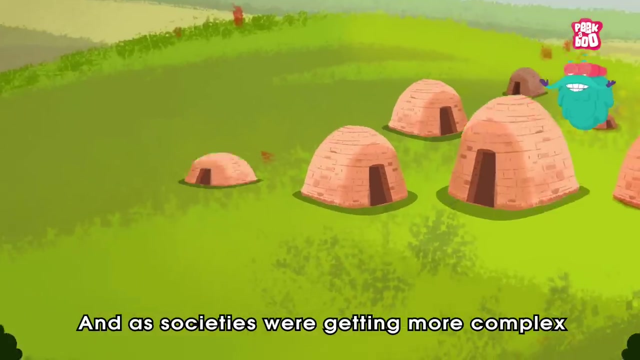 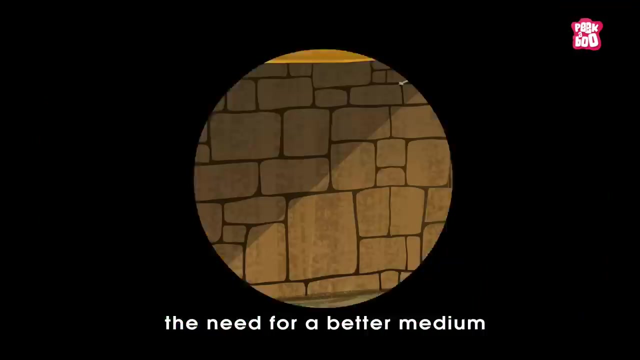 in most cases, But unfortunately it has many limitations, as not all goods or services were easily traded and there was no easy way to determine the value of goods or services, And as societies were getting more complex and people were traveling around the world, the need for a better medium of exchange became a necessity. 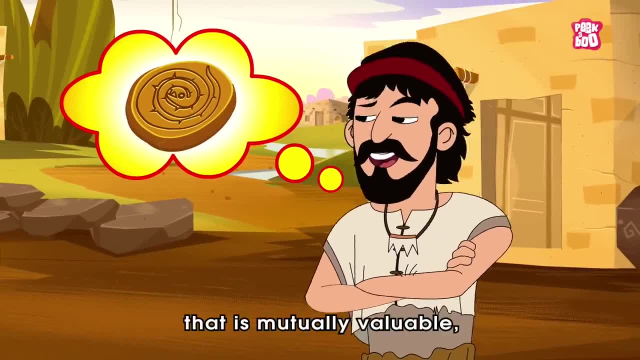 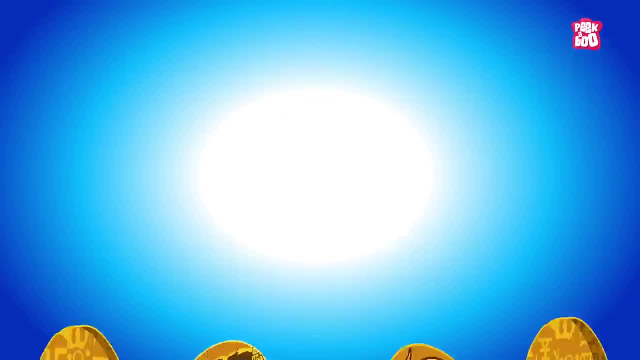 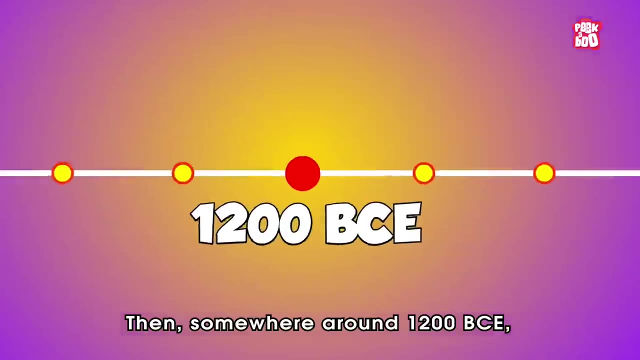 People understood that they require something that is mutually valuable, can be easily calculated, can be reproduced and can be stored for a long period of time. Then, somewhere around 1200 BCE, many ancient cultures began to use things like gold, silver and silver to trade their goods and services. 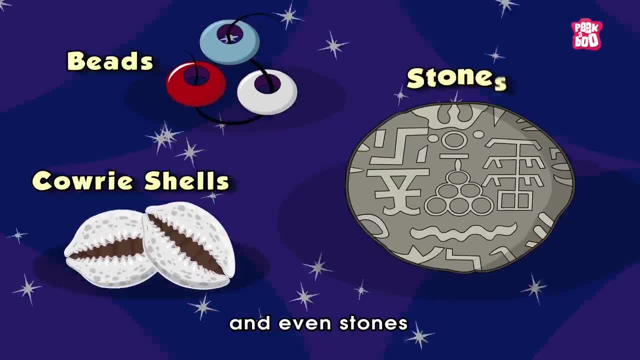 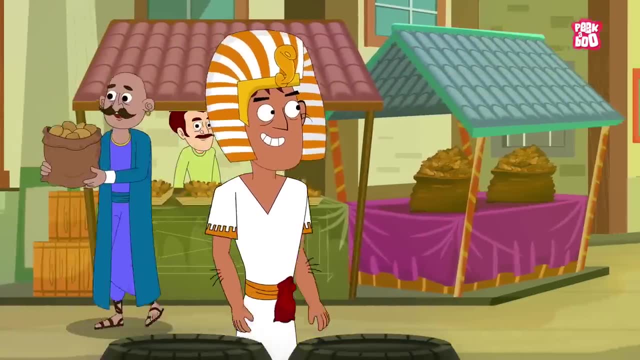 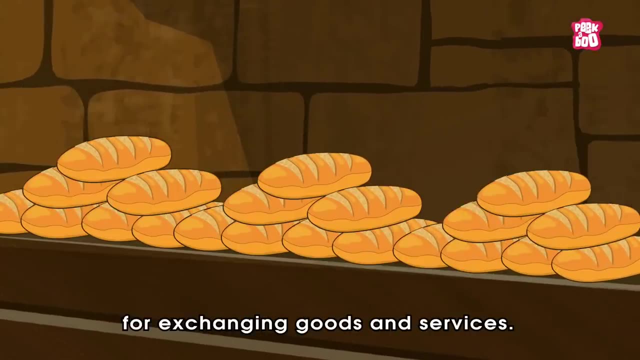 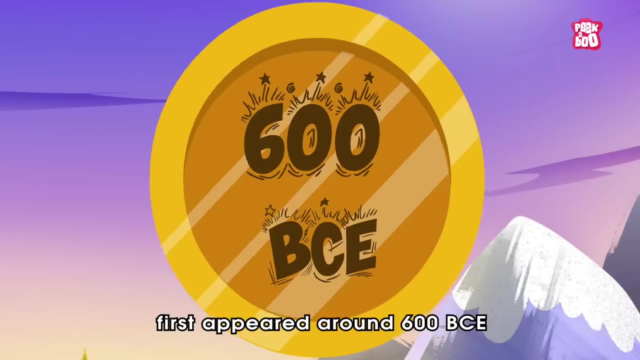 Like cowrie, shells, beads and even stones. as an early form of money, These items were small, portable and easy to trade. Plus, they had a consistent value which made them ideal for exchanging goods and services. But metallic coins as we know them today first appeared around 600 BCE in a region called Lydia. 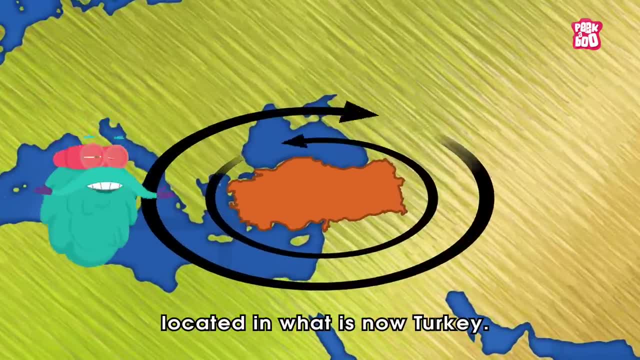 an ancient kingdom of the Roman Empire. This region was known as the Roman Empire. It was also known as the Roman Empire. It was also known as the Roman Empire, Located in what is now Turkey. these coins were made from a mixture of gold and silver. 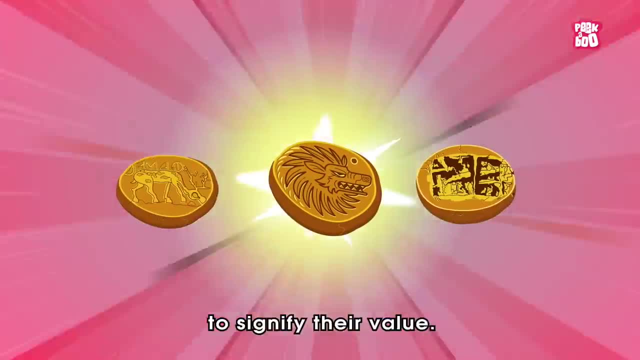 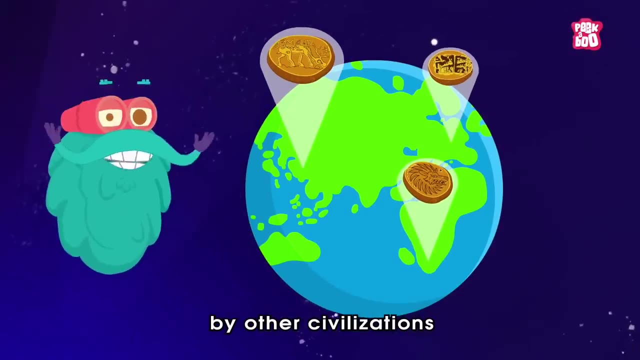 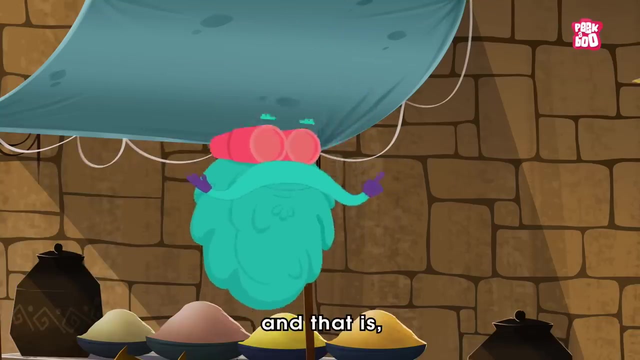 and were stamped with various images and symbols to signify their value. Soon, coins became popular and were adopted by other civilizations throughout the world, But there was still a tiny viney problem, and that is too. many of them were quite heavy to carry. 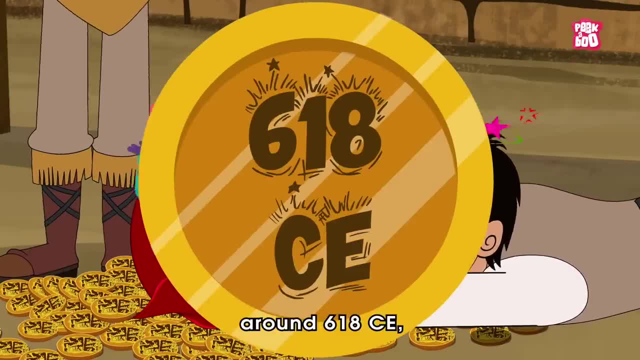 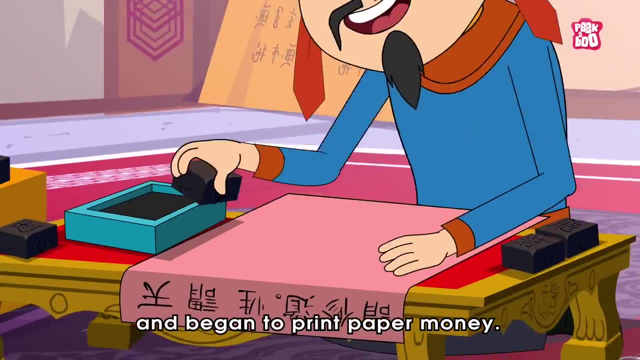 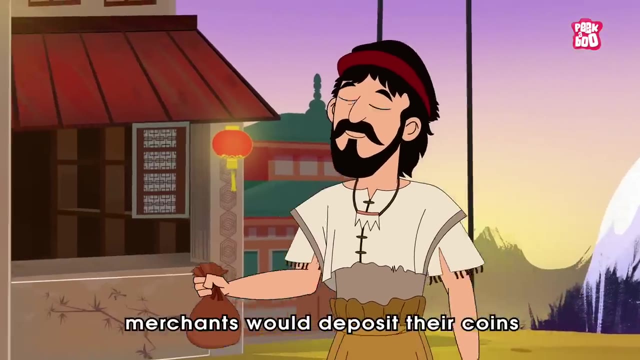 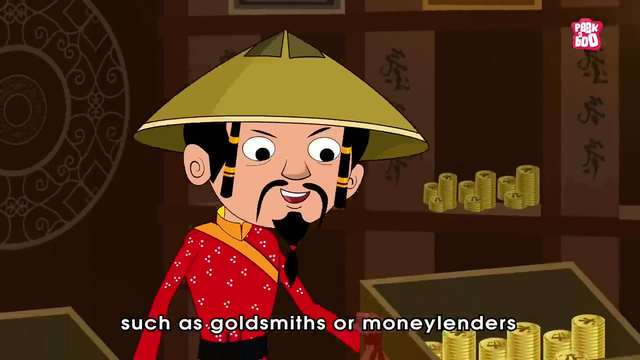 So to tackle this weight around 618 CE, the Chinese thought of making the most out of their invention of paper and began to print paper money. At that time, merchants would deposit their coins with trustworthy individuals such as goldsmiths or money lenders, and receive a paper receipt in return, which they